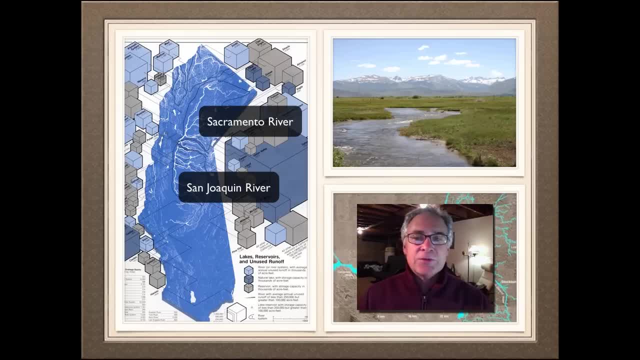 meadow picture, you'll see that there's a lot of streams and rivers in the spring, with snowmelt coming off of there to also recharge some of the smaller watersheds. But if you take a look at the vast network of needs in our state, as pictured here on the left, you'll notice that there are 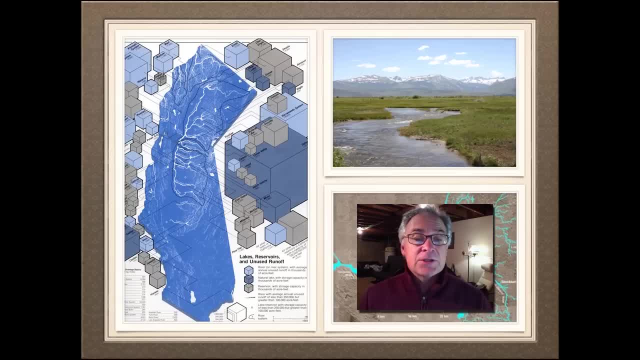 all different kinds of water districts, Also municipalities, a huge system of levees and dikes and, of course, dams all over the state to control our waterways and control the amount of surface water that runs through the state. But again, as we control the surface water, we can also control the groundwater as well. 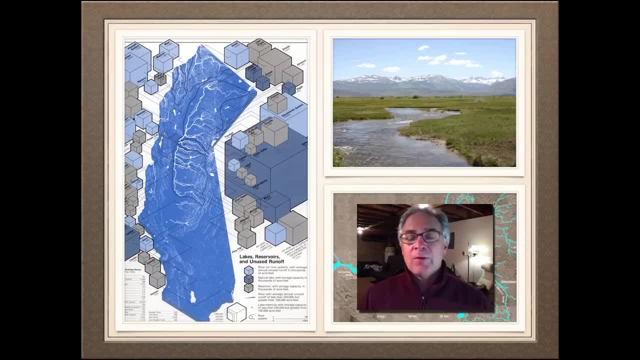 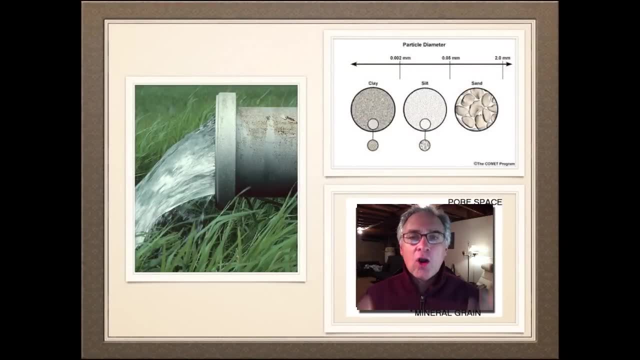 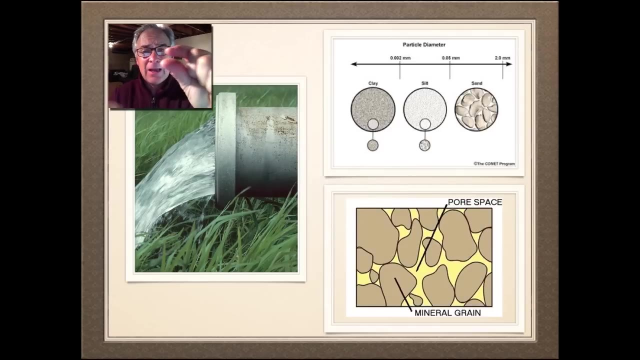 so that it can be recharged not only for drinking water but also agriculture as well, And kind of the workhorse of all of this maintenance of our groundwaters and our aquifers is really a little bitty tiny guy. He's about even smaller than that, sometimes even microscopic, And those are called. 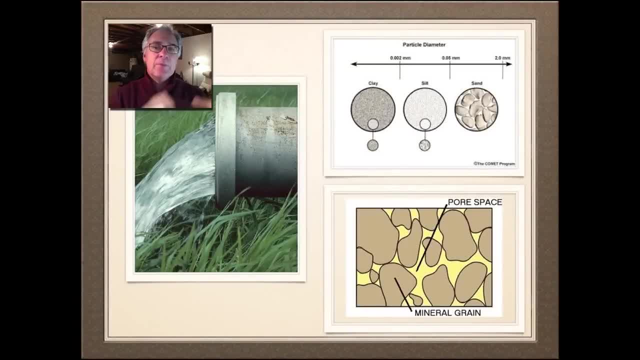 pore spaces. Pore spaces are the space in between the soil particles. So before we can even pump water out of the ground to irrigate, like this picture depicts, what we have to do is manage that pore space. Those little bitty pore spaces are vital to the water supply of the state. 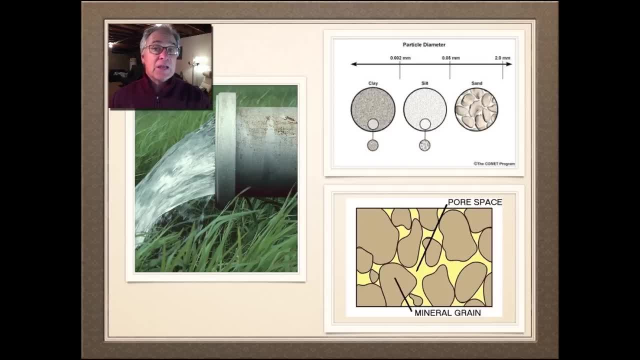 These are called pore spaces, and the only ways we can manage it is to basically pull it up and leave it. They are called pore spaces. You know where they come in and out? Well, joy parks. Yeah, Yeah, I love it. 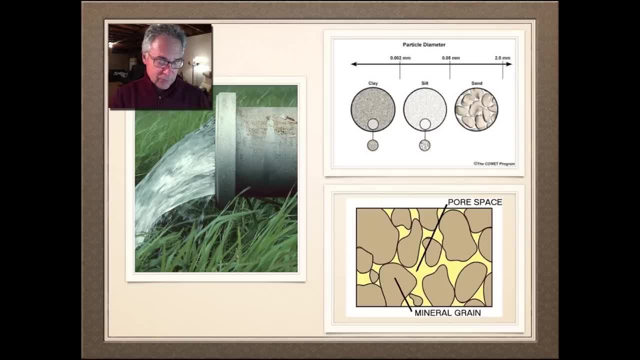 Yeah, I love it. It had guys lengthen them 25, 60 meters. It had chybacs on them. you know. conclude them, Let's go on. Yeah, that's quite cool. I got the same size is how I'm gonna determine if this area is beneficial in all the aquifers. 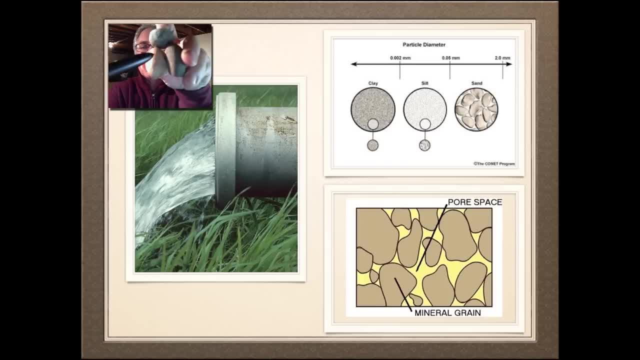 Whether it be sand, silt or clay, they have different sizes and, of course, the different size will lead to the amount of water which a particular unit of volume of soil can hold. artistic手多力 cancer nationale. If these are three particles. if you notice right there in the center, this hole is called. 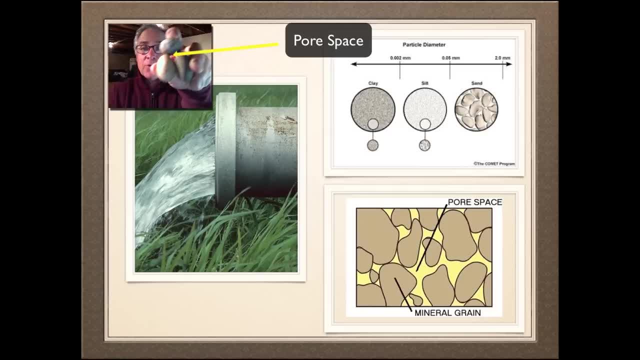 a pore space. That's the part in a soil matrix that's either filled up with air or water. If it's an aquifer, it's probably filled with water, or at least most of the time anyway. As the water table will fluctuate in one of the aquifers, it will be filled up or taken. 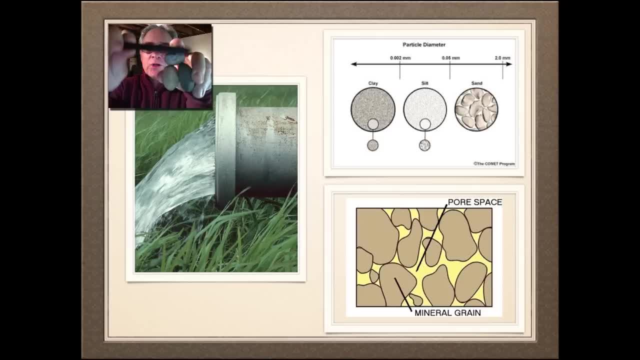 away, depending if it's pumped out or it gets recharged by some kind of source. So these three particles right here are, of course, the soil- mineral, if you will, and this right here would be, of course, the pore space that fills with water. 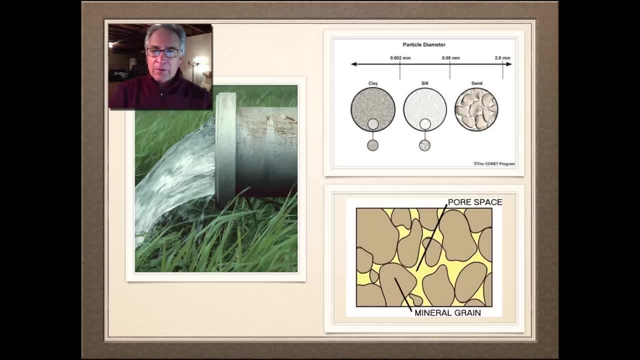 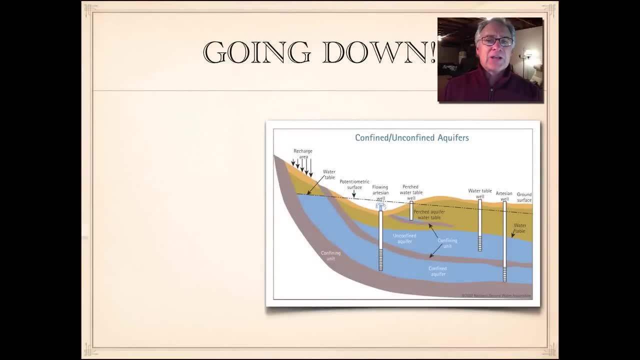 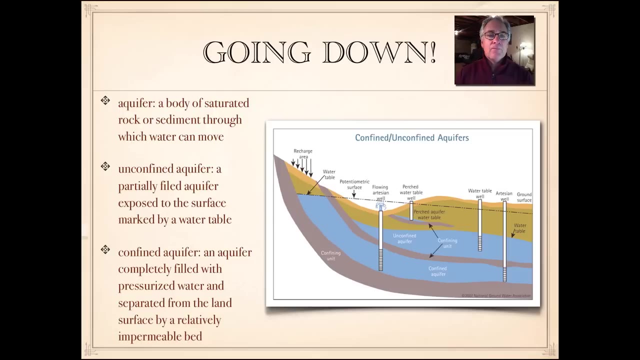 So that kind of gives you an idea what kind of the workhorse of the aquifer is. and that's that pore space Now for water to actually go down into the ground and percolate down into the soil. when that happens, then we have an aquifer. 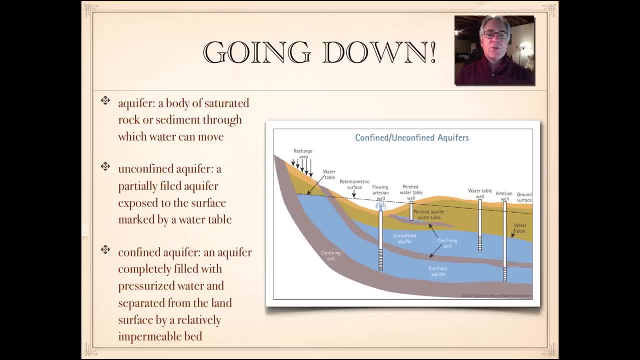 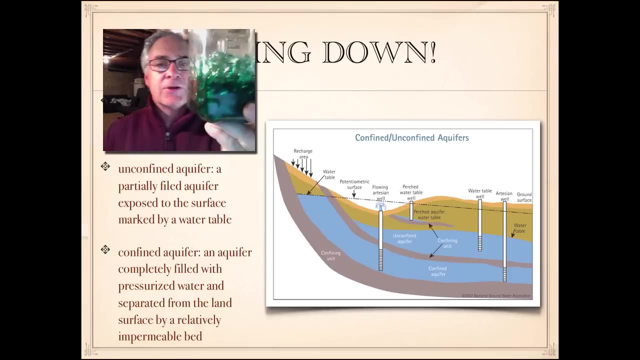 Now, as water fills up those tiny little pore spaces and fills up that particular area of soil, then what we do have is we have an aquifer- And I brought along a model here today to kind of show you that- And here's our model of our aquifer. 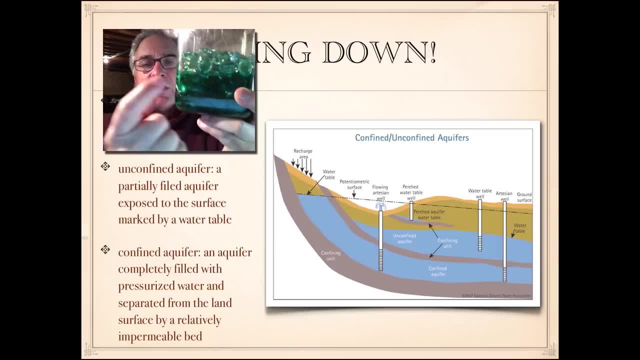 You notice that this represents all the little glass beads in here are going to represent soil particles. The green water in here shows you where this water has settled. Because of this kind of confining layer on the bottom, the soil can't go any further. 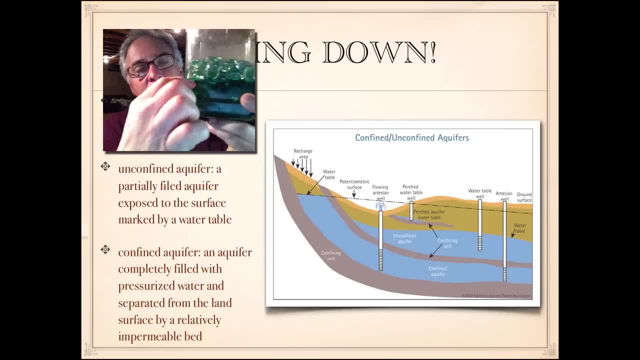 Let's call that clay, for instance. So if we were to take a look at where the water table is, or the level of water in this aquifer that's called the water table, you'd see it at 600 milliliters. 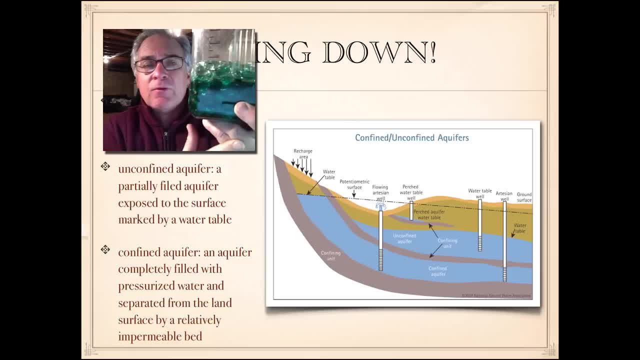 And with that in mind, that looks like there's a deterministic amount of water. But we have to also consider: in an aquifer it's this kind of this body of saturated rock or sediment in which water can kind of move in and out of. 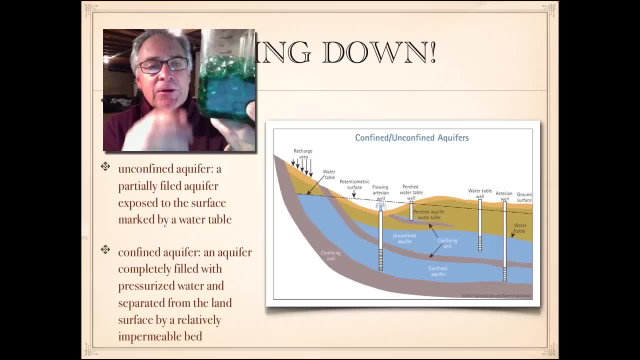 And of course you can see as I turn, this water can move through it. So these pore spaces are large enough to allow that to take place. But how much water can this aquifer hold? Well, one way that we can determine that is by determining the percentage of pore space. 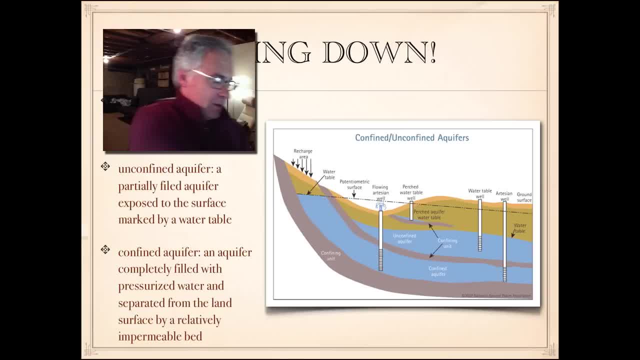 or porosity. So I'm going to go ahead and pour this water out, And as I do that, we'll be able to somewhat calculate about what the pore space is. So what I'm doing is trying to keep all the rocks still in place. 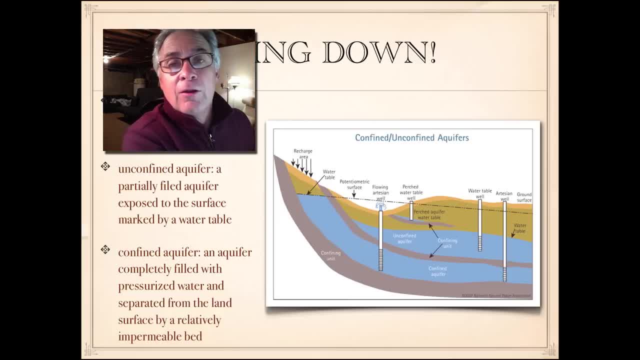 Okay, I'm pouring out all the water as much as I can, But notice that even though I pour it all out, some of it still sticks to all the soil particles. So even though you can drain it, there is still left some water in between these pore. 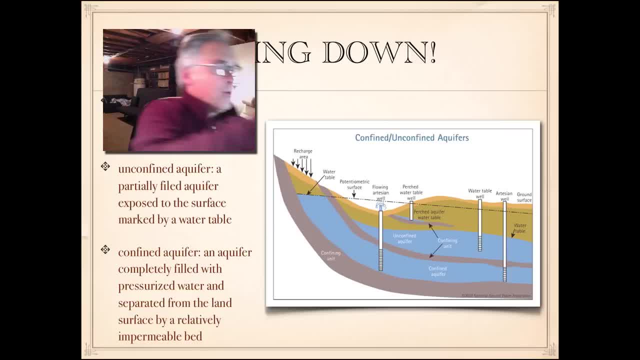 spaces It doesn't always, ever leave. So when I poured it out, you can see that we have just about 300 mLs, Roughly about 50% pore space, And of course in the real world that's probably not a really good example of that. 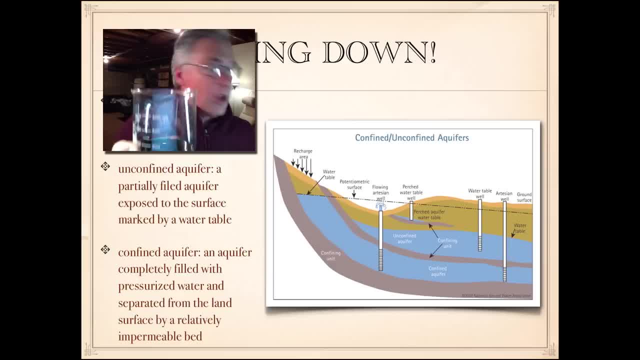 But it just gives you an opportunity to see that even though it looked like it was 600 mLs, a lot of it was. the room was taken up or the volume was taken up by the actual matrices of the mineral or the mass. So an aquifer is kind of like this sponge. 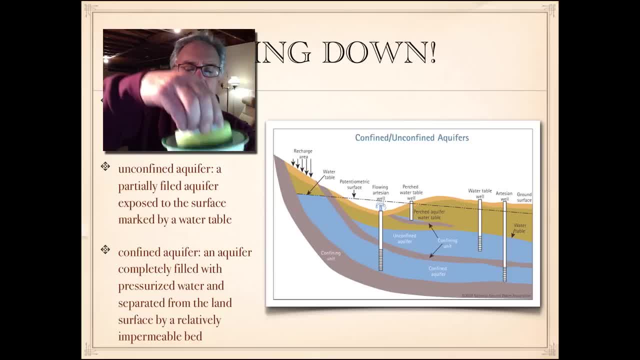 It will soak up water And hold it there. But if we were to kind of squeeze it, you can see that in this sponge it's of course spread out And what's being filled up in this sponge, That's right, The pore spaces. 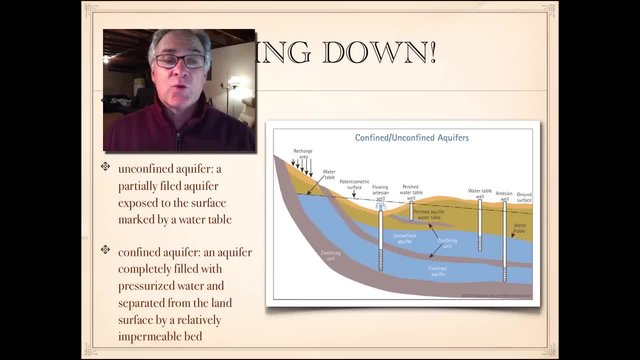 So again, an aquifer is just a body of saturated matrix, in particular of rock or some kind of sediment, in which water can flow through. It can be easy to go through or hard. Now, when we look at the aquifers themselves, they're different types. 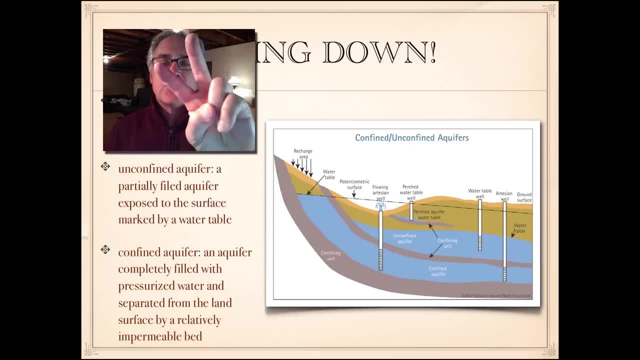 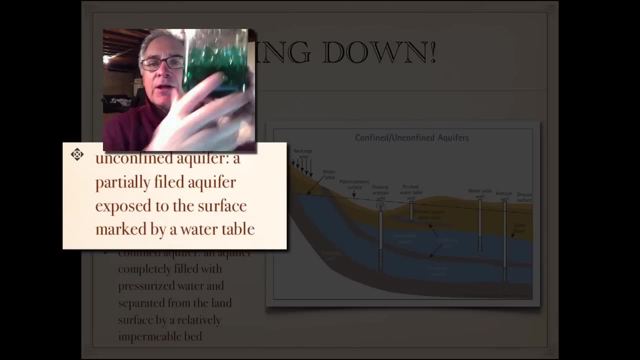 Okay, We're going to talk about just two of them, And the one that you'll see on your groundwater model most probably are these two. The first one is called an unconfined aquifer, And the model that I showed you today is a good example of an unconfined aquifer. 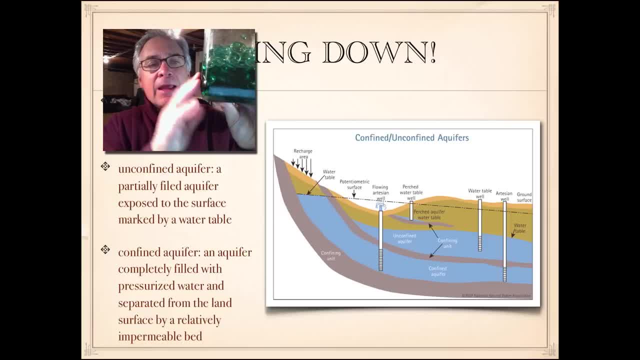 This unconfined aquifer basically is open access to the top layer of soil. Maybe on the bottom there is something confining it, But for the most part It's just partially filled with water. You can see that we still have a little bit of what they call headspace, where this water 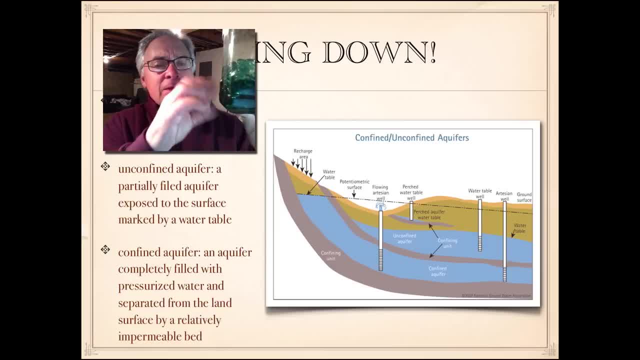 table is, And that means this aquifer isn't completely filled And it is exposed to the subsurface marked by this water table right here And because it really doesn't have any confined layer or it doesn't really have anything pushing down on it, it's basically unpressurized. 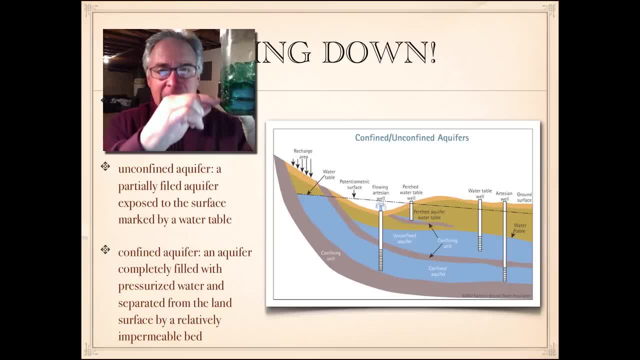 So water will flow in and out. This water table will go down and up depending on the season, depending on how much it's used as far as the pump is concerned. So that's an unconfined aquifer, If we take a look at our drawing here. 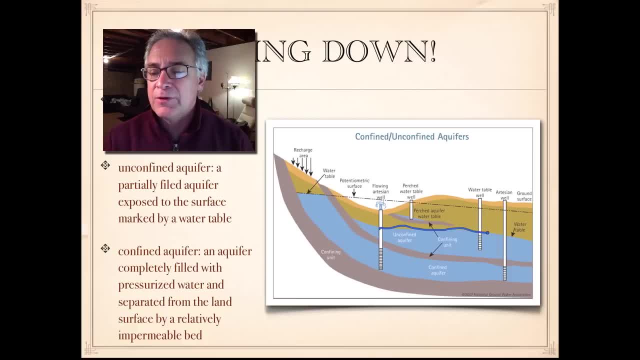 This is the water table right here on this unconfined aquifer, And it's exposed to the open surface right here And it does kind of have a confining unit to it. In other words, here is a confining layer of clay. 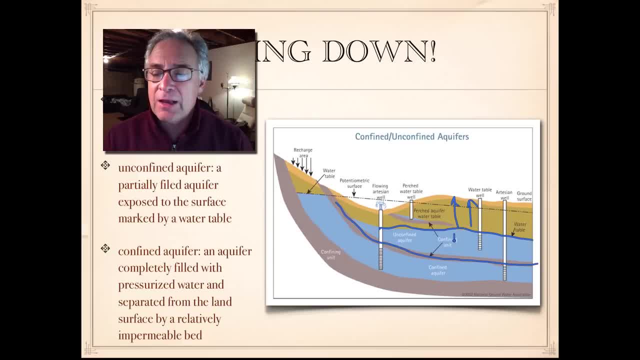 And of course it can't go all the way down, So it fills up as it gets recharged from a river or a lake or even rain itself. So that would be an unconfined aquifer. Now we have a different kind. Let's suppose again using this model, if there was another aquifer beneath this plastic. 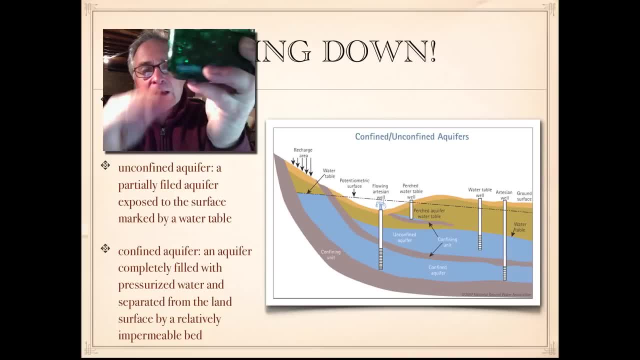 we'll call this clay, just for lack of a better model. anything underneath this would be considered a confined aquifer Because it's confined at the top, Whereas this was unconfined at the top. A confining layer or a confined aquifer is confined not only on the top, but also on the. 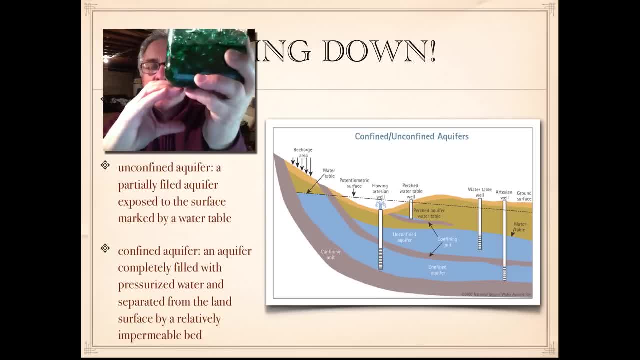 bottom. So it's pressurized, It's always filled up. So in a confined aquifer situation it's always filled up. number one. Number two: it's under pressure. So if you've ever traveled the mountains and taken a drink from a spring, you'll know that. 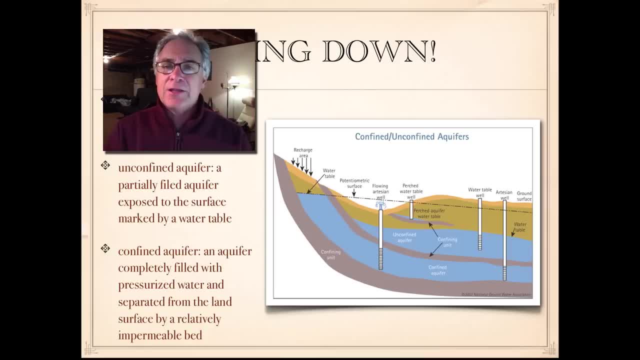 it seems to just continue to kind of pour out, And the reason why it does that Is there's a fracture or a break in that confining layer, so that it actually scoots through that fracture and of course it's under pressure, so it's kind of leaking out under pressure. 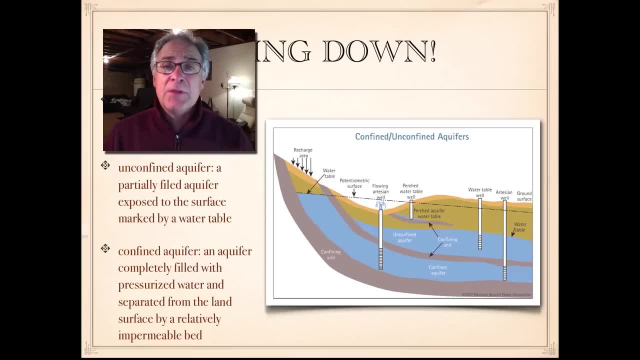 There's two reasons why it's under pressure. Number one: it's being recharged from a different place. So again, if we take a look at our diagram here, here's a recharge area for the confining aquifer, or confined aquifer. 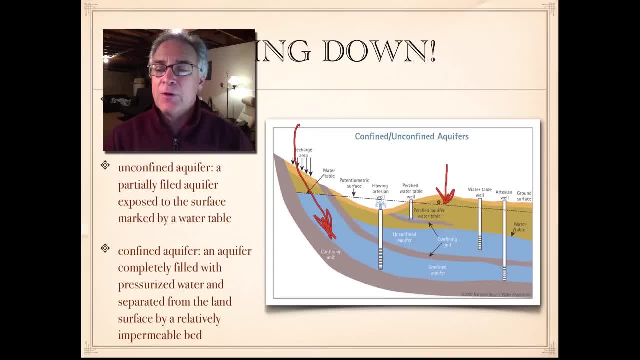 Whereas, of course, on the unconfined aquifer it's just located right over top of the- you know the aquifer. So this one has two confining layers, one on the top, one on the bottom, And this tends not to empty. 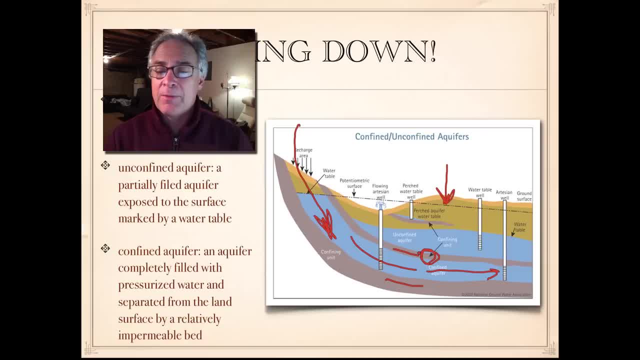 Because if it did, then of course all of this would come probably crashing down and you'd have what we call subsidence: The water, the area or land around it would sink. We see that in the southeastern part of the United States from time to time, as we have. 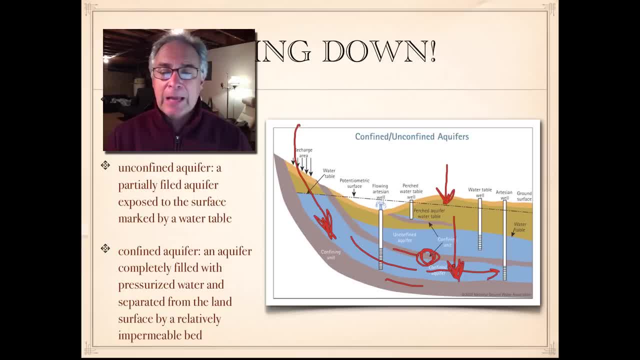 these big sinkholes, And that's typically what happens. So the recharge area for the confining aquifer, So that's what we call subsidence- The water will sink. The confining layer is different than the one on the unconfined layer. 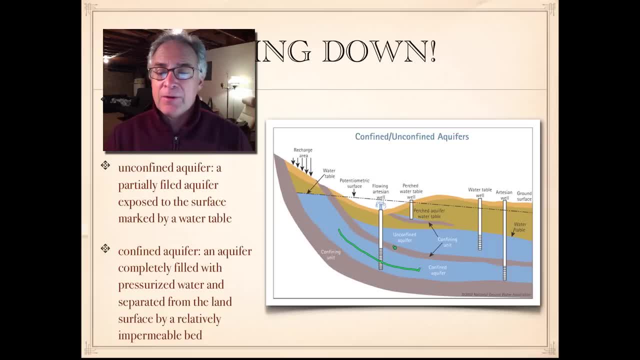 So again we have a confined aquifer that is surrounded by essentially two confining layers, Typically of clay or bedrock or shale or some kind of impermeable layer that you know water can't get through very easily. And then we have also the unconfined aquifer right here. 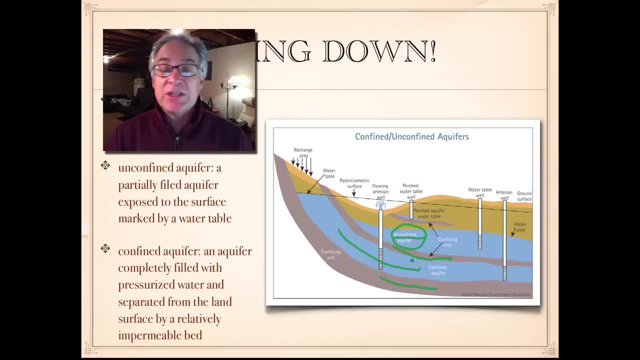 And that is open to the surface, Whereas this one is not. It's enclosed, It's sealed, if you will. So it's under pressure. So if there's a fracture or a break, like right here, water can come through here as a spring. 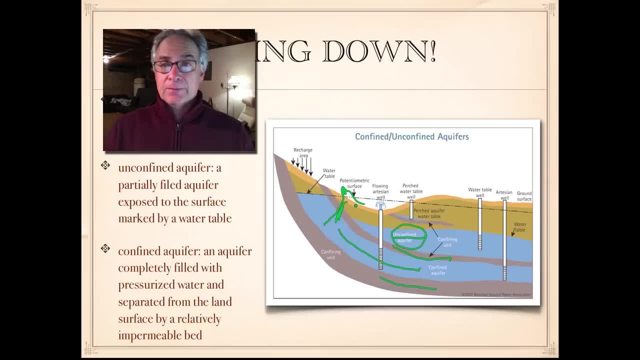 And then, of course, it would run down the hill and maybe form a small stream ponds wetland area. what have you? So those are the two kinds of aquifers we're looking at: confined and unconfined. Basically, the difference is: unconfined is open. It's not pressurized. The confining layer has basically two different kinds of impermeable layers surrounding it to keep it under pressure. It doesn't fluctuate much- A little bit, but not much- Whereas the unconfined fluctuates a lot. 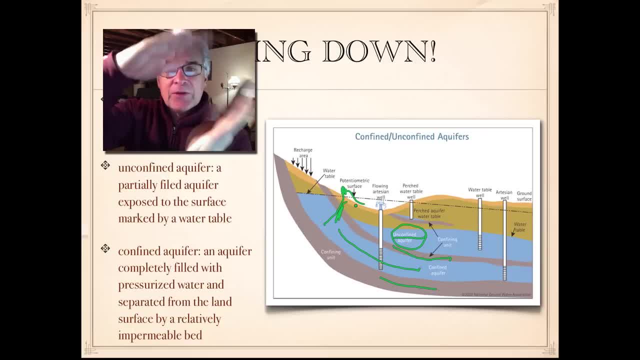 Well, I hope that helps. Please make sure you see the other two videos on the basics of groundwater, And those should help you with your lab over the next couple of days. We'll be back with a new video soon, So until then, thanks for watching. 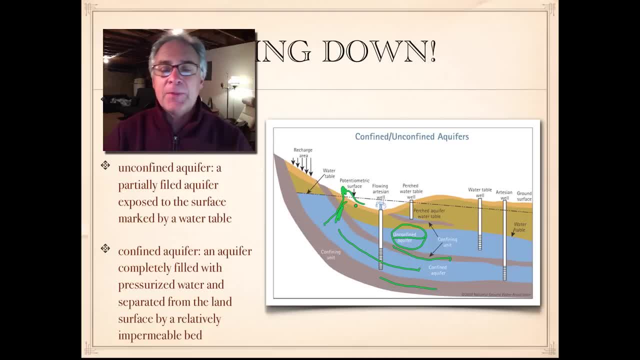 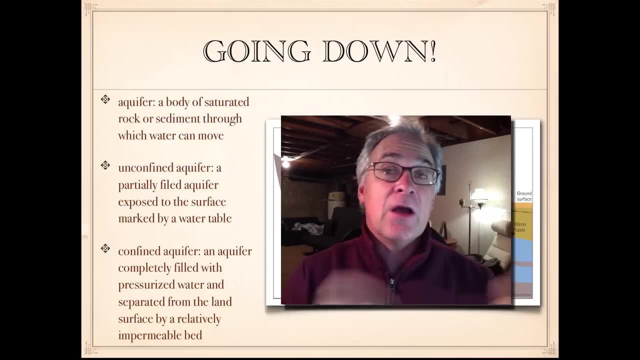 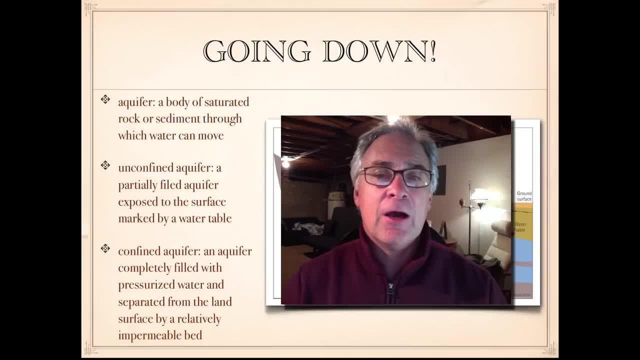 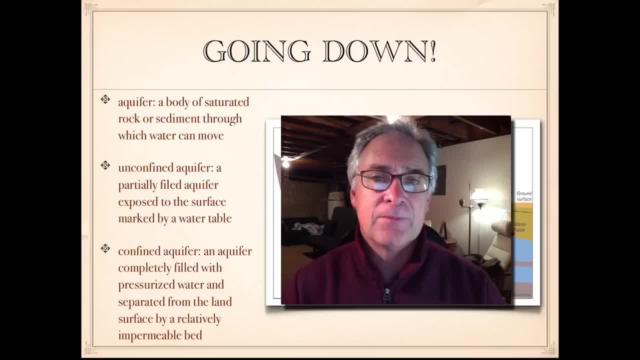 We spent some time with the Somnod. I think it was either a big and it was a small short video. Cheering, similar to my last video was much more affordable compared to the long video that you've seen. Thank you everyone. 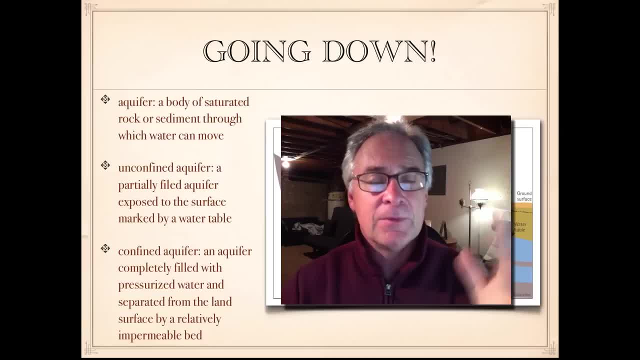 Thank you, I hope that. thanks for watching. See ya, Thanks See ya, Bye. Good luck with the videos up next. Check that out later. Okay, Feel free to review some YouTube interviews that I've posted, If you have any question here about the demarcation items. thank you for watching. See ya.